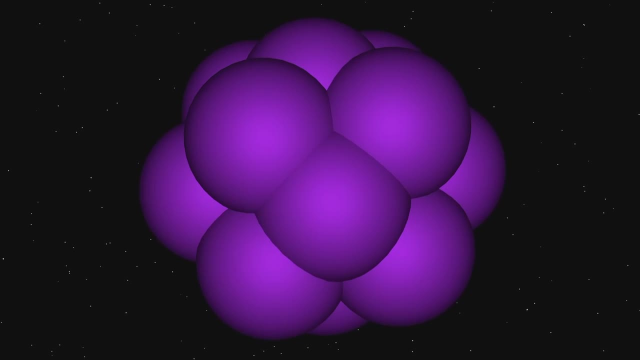 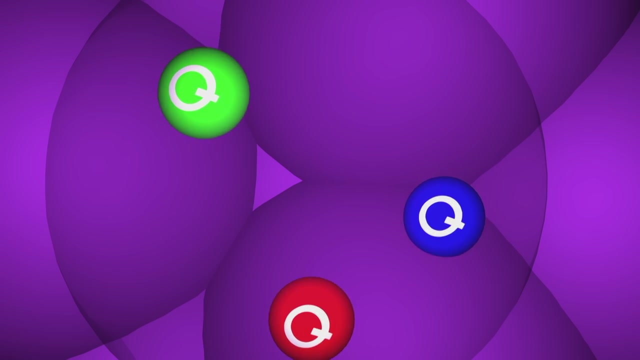 with. we know that the tiny protons and neutrons at the center of atoms are made of even smaller particles called quarks. Quarks were proposed in 1964 and proven to be real in the 1970s. The existence of quarks is well established. 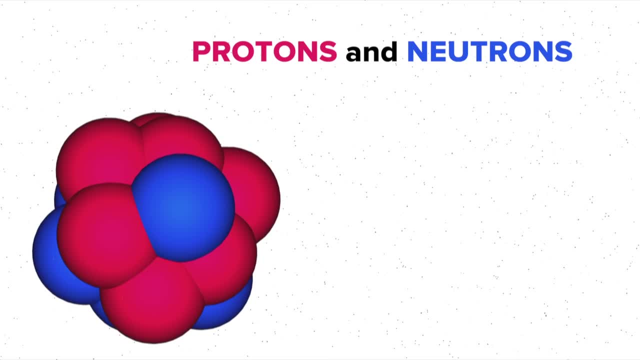 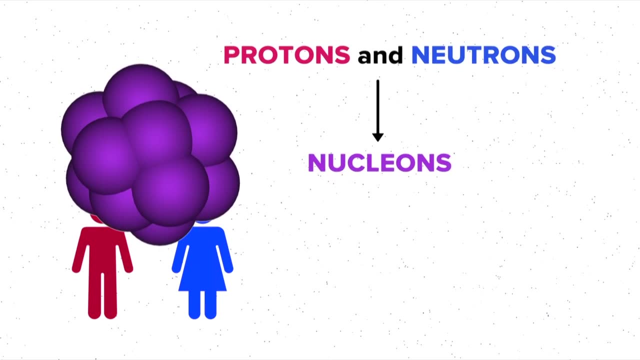 science. Because protons and neutrons are found inside the nucleus of atoms, we call them by the overarching and generic term nucleons. That's basically like how we can distinguish men and women and yet combine them too and call them by the single term human. 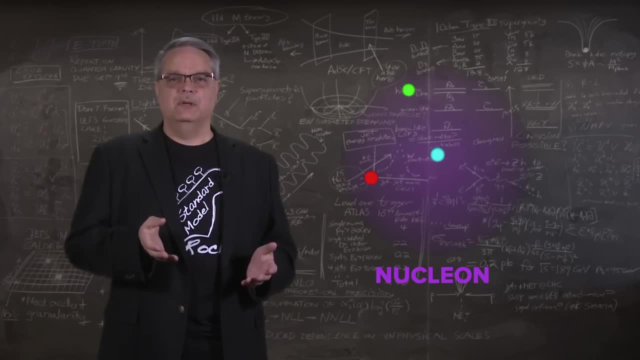 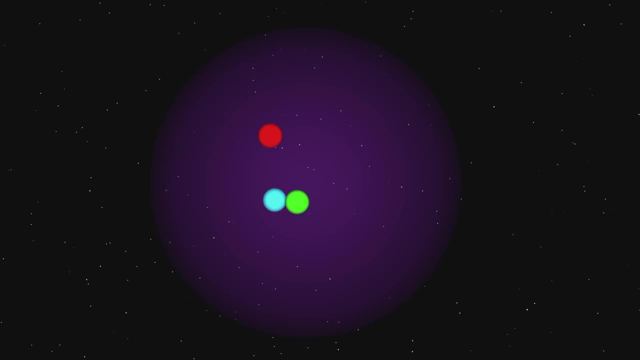 Each nucleon consists of three quarks. That's a simplified picture of what's going on inside, but it helps us understand the key points. You can think of a nucleon as a tiny sphere with a radius of about a quadrillionth of. 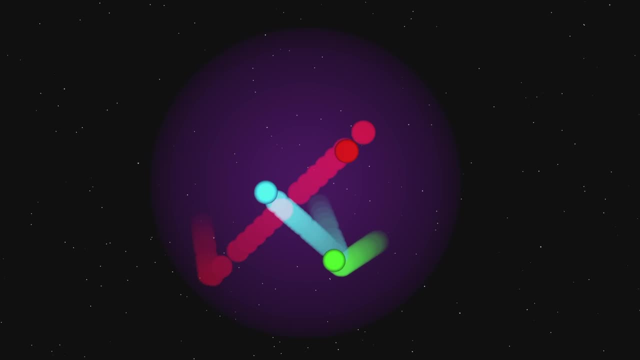 a meter across The quarks, zoom around inside the sphere, traveling at nearly the speed of light. And if you have particles moving at that outrageous speed, in that ridiculously small volume, you have to have an ultra mega strong force holding it all together. And 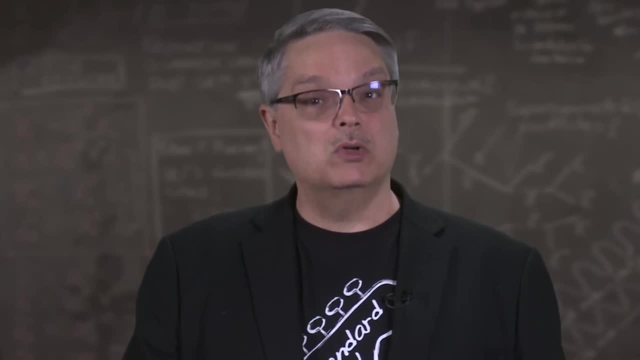 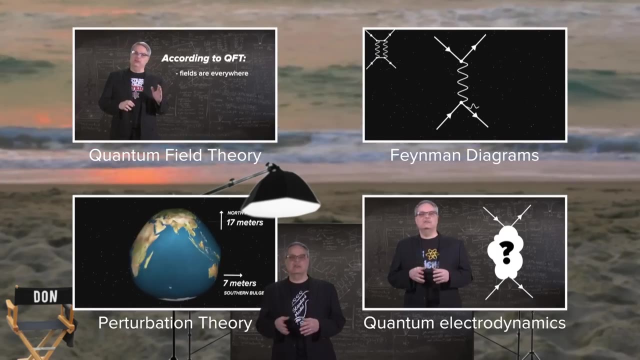 because we're talking about the realm of light. we can't just force a quark in one realm of the super-tiny. the force governing the motion of quarks has to be a quantum force. Now I've made lots of videos on quantum forces, If you're interested in the subject. 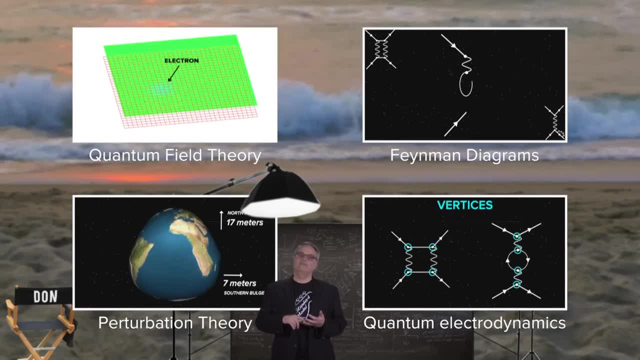 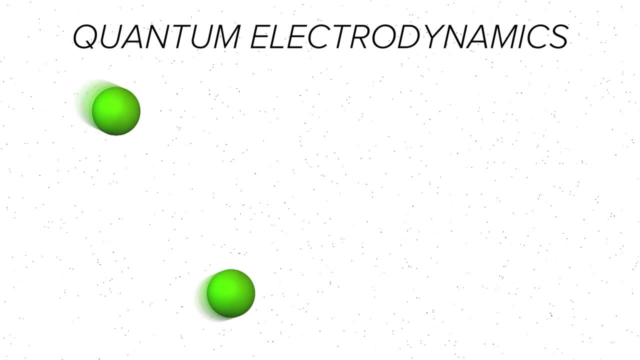 matter. I recommend watching four other videos on quantum field theory: Feynman diagrams, perturbation theory and quantum electrodynamics. But I can give you the high points here. The simplest of the quantum theories is called quantum electrodynamics or QED. That theory 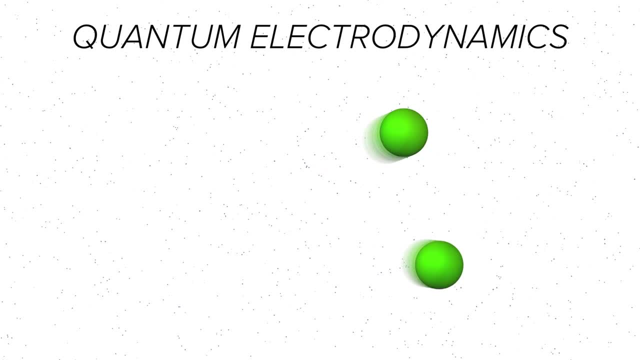 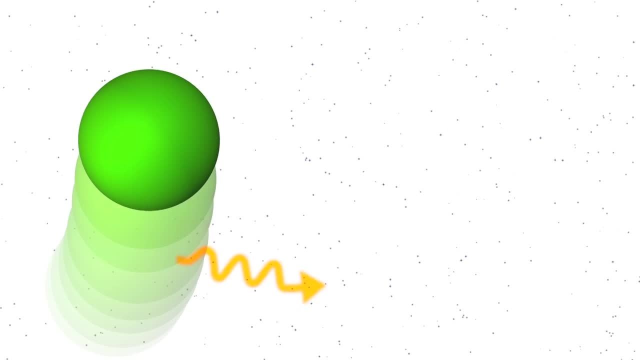 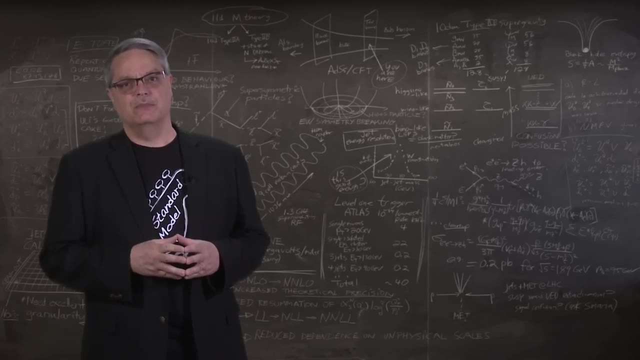 talks about how electrically charged particles interact by shooting photons back and forth between each other. The simplest interaction occurs when a charged particle like an electron emits a photon and then recoils. Now the force holding the quarks inside nucleons work a little differently. First the relevant 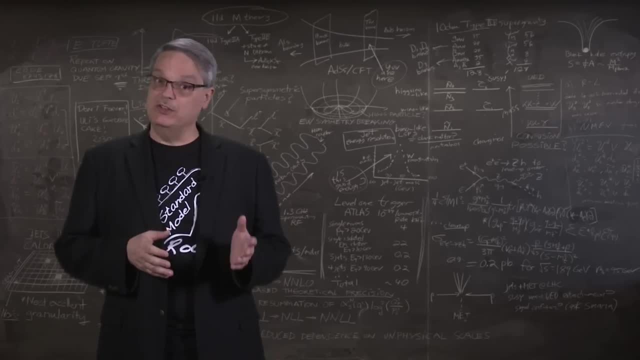 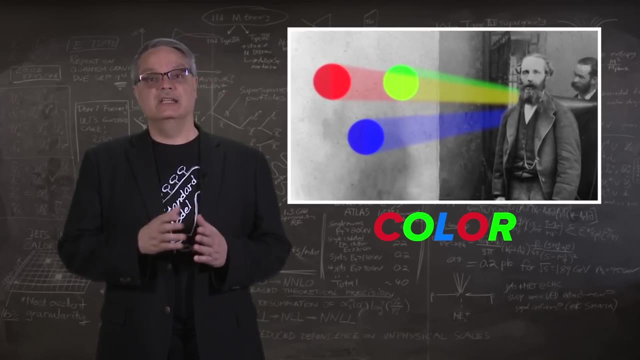 charge is not the electric charge, but the strong force charge, what physicists call color. I talk about quantum color in yet another video, but color in this context is basically a different kind of charge. It has nothing to do with color in the normal sense of the. 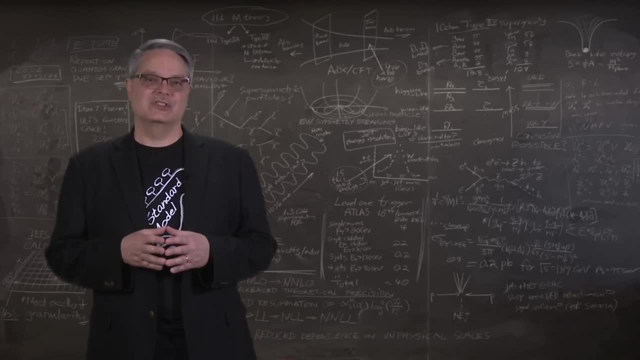 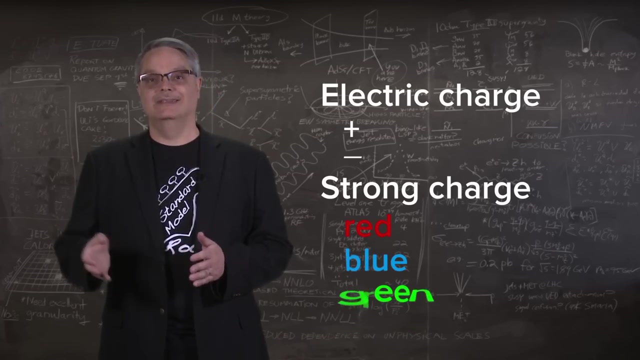 word. Sorry about that, by the way, My tribe of particle physicists do have an idiosyncratic way of naming things. In any event, unlike electric charge, which comes in two varieties, plus and minus, the strong charge comes in three varieties, named red, blue and green. Again, nothing to do. 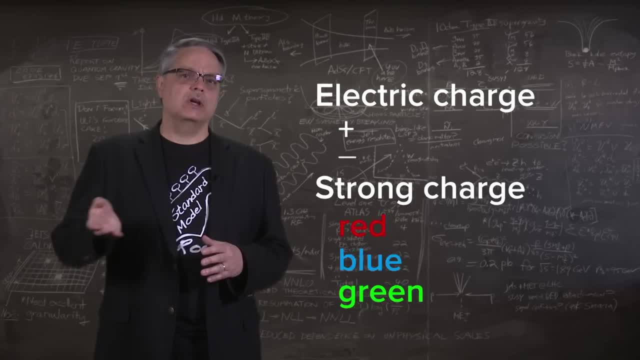 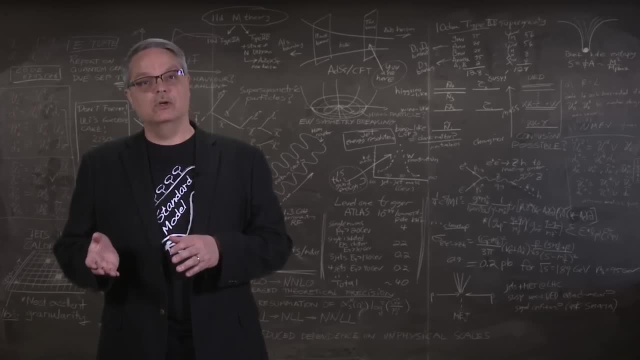 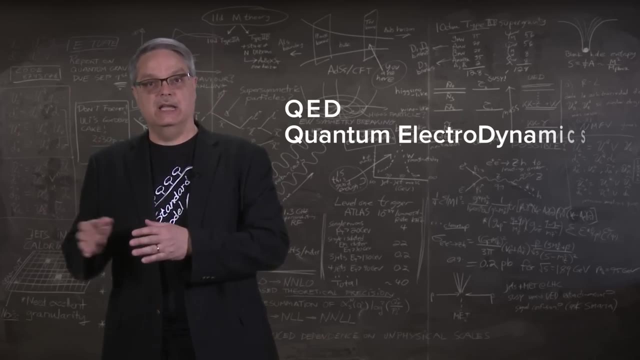 with regular color. The particles that the colored quarks exchange are not photons, but rather particles called gluons. The photon is the particle of the electromagnetic force and the gluon is the particle of the strong force And in analogy with QED or quantum electrodynamics we call 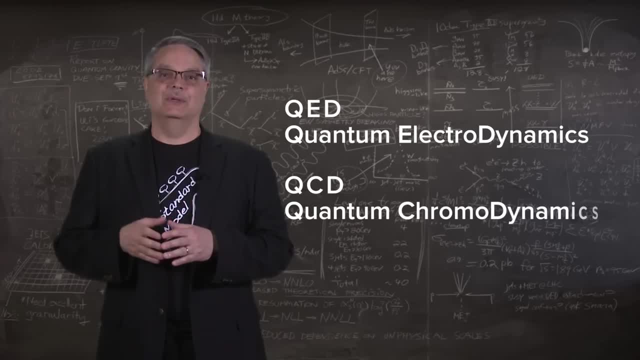 this theory, QCD for quantum chromodynamics. Get it Chromo color. Sometimes I'm a little embarrassed by my tribe. For those of you who are fans of Feynman diagrams, we draw an exchanged photon as a wavy line. 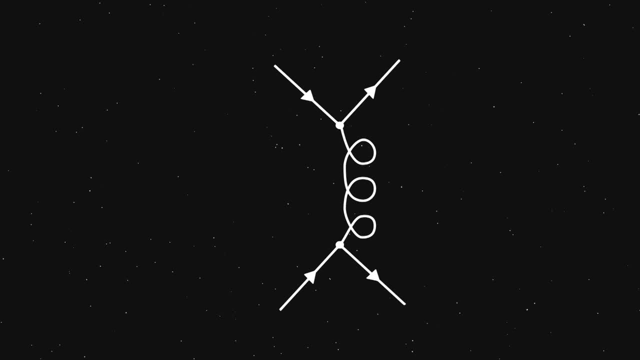 while a gluon is a corkscrew. And, just like all Feynman diagrams, the Feynman diagram of two quarks exchanging a gluon corresponds to an equation that a sufficiently diligent student can solve, But it's pretty hard. so kids don't try this at home. 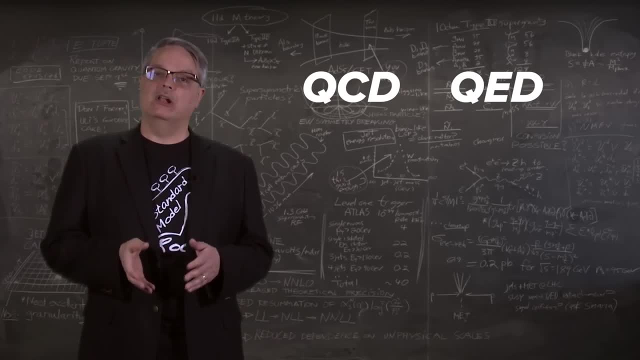 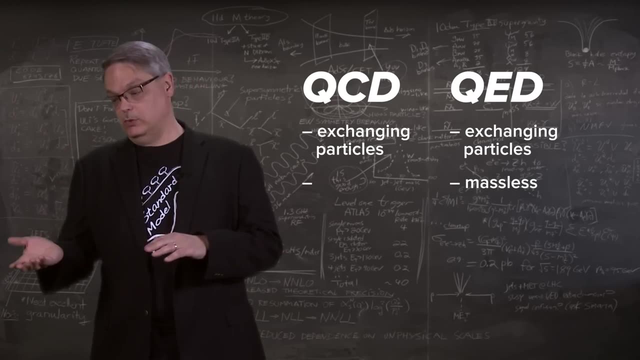 So how is QCD different from QED? Both involve exchanging force-carrying particles between other particles carrying charge. The photon is massless, The gluon is massless. The photon has no electric charge, The gluon has no. Oh wait, wait. 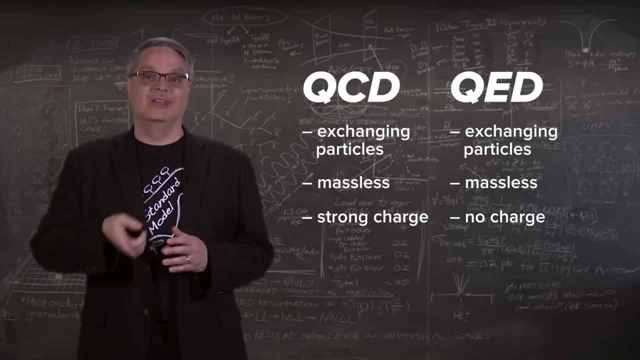 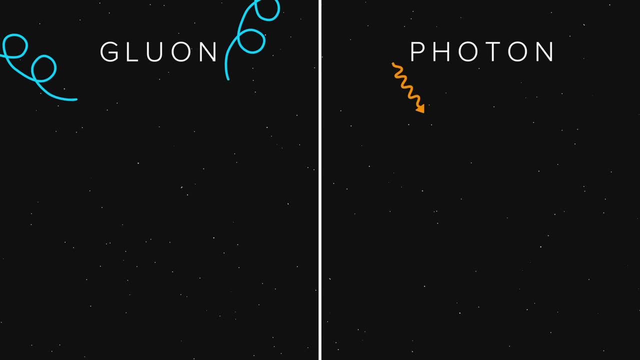 Wait a minute. There's a difference. Gluons carry the strong charge, They have color, And that little difference has a huge consequence Because gluons interact with colored particles. gluons can interact with other gluons. That's way different than two photons, which are 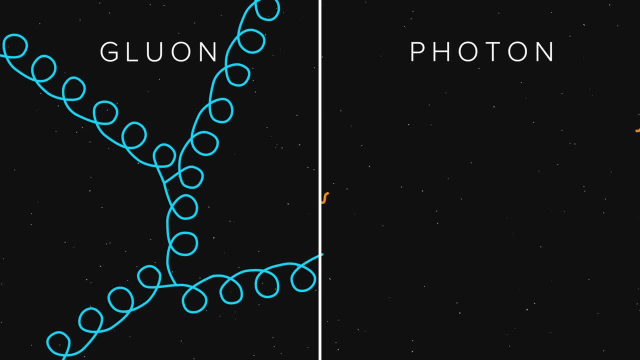 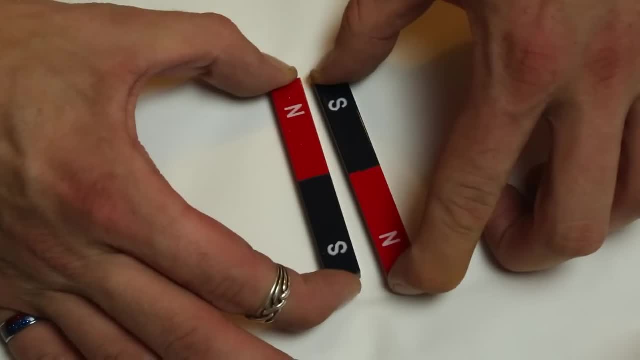 completely oblivious of each other's existence And it qualitatively changes the behavior of the strong force. Let me explain. If you have two magnets and kind of play around with them, you quickly find out that they feel a stronger force between them if they're close to one another and a weaker force if they're far apart. That's how the electromagnetic force works. On the other hand, if you have a rubber band, you find that the two ends don't feel much of a force when the band isn't stretched, But as you stretch it the force gets stronger.